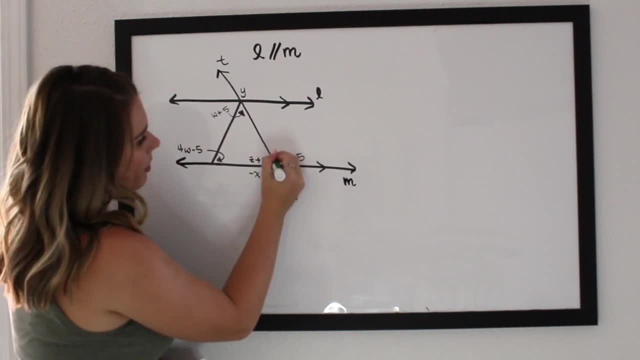 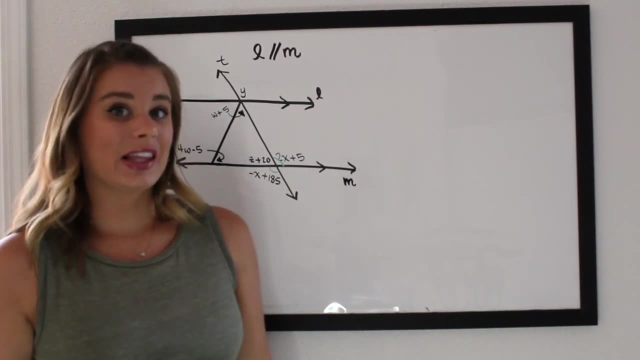 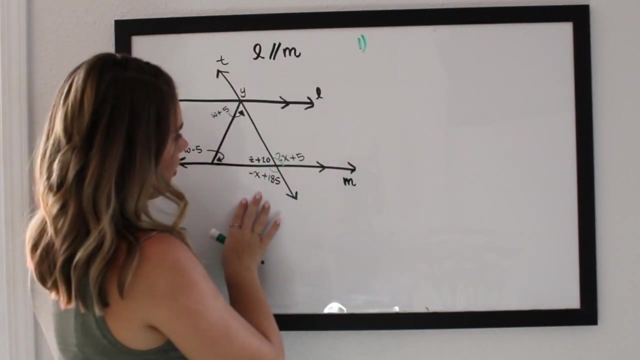 kind of jumps out at me looking at this diagram is: I have a pair of vertical angles, So what we need to do is state the theorem we use before we write the equation. So my first equation is going to be the theorem that vertical angles- and this is how I abbreviate it- are equal Vertical. 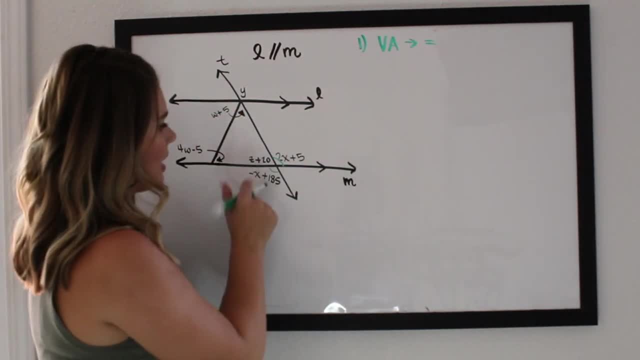 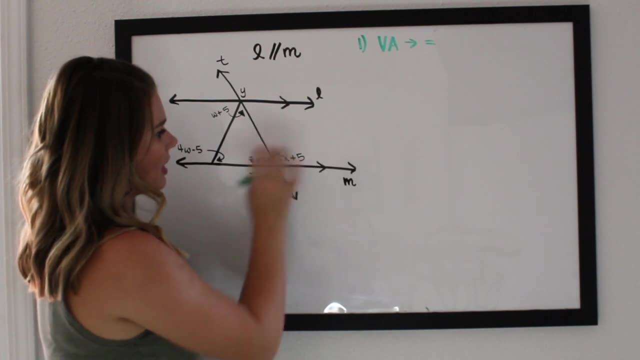 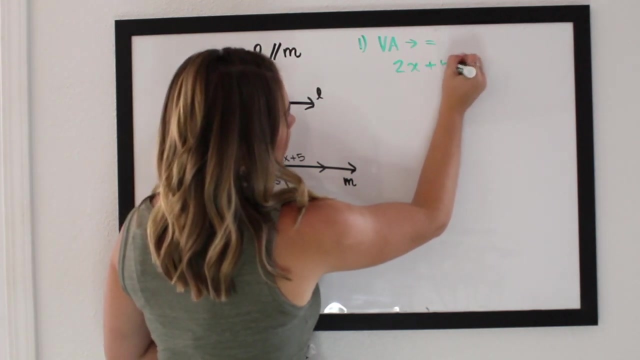 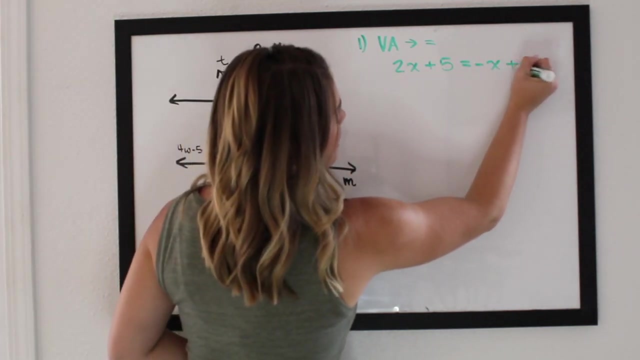 angles therefore equal, And so that means this angle is equal in measure to this one. So negative X plus 185 is going to equal 2X plus 5.. So 2X plus 5 equals negative X Plus 185.. I'm going to solve this in black just because it's a little easier for you to see on. 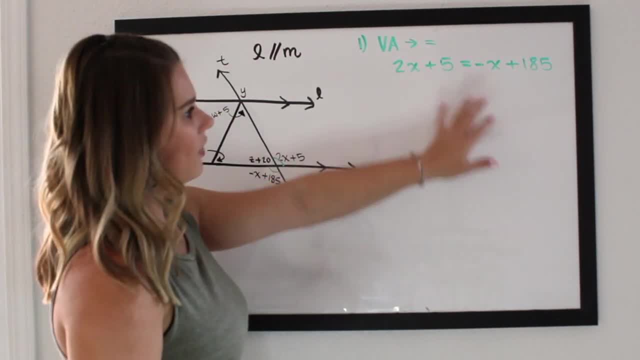 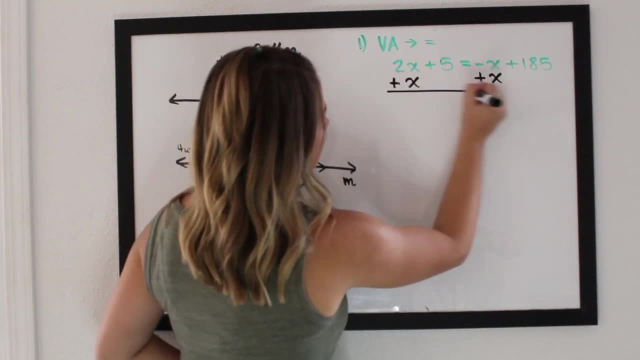 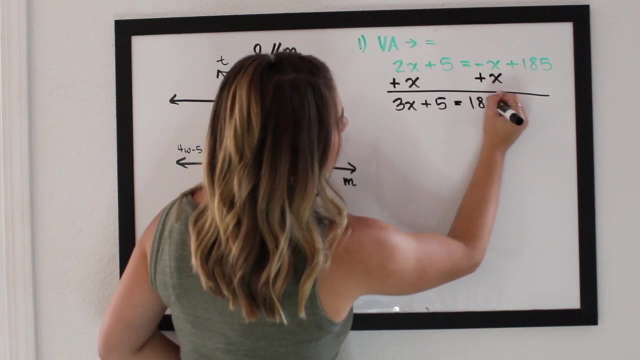 camera. Okay, so now I need to solve this thing for X, So I'm going to add X to both sides. I end up with: 3X plus 5 is equal to 185.. I'm going to subtract 5 from both sides. 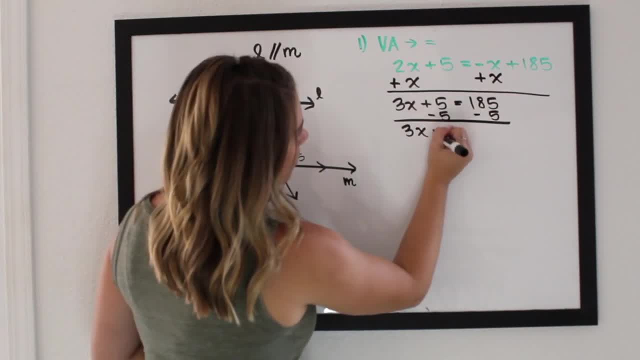 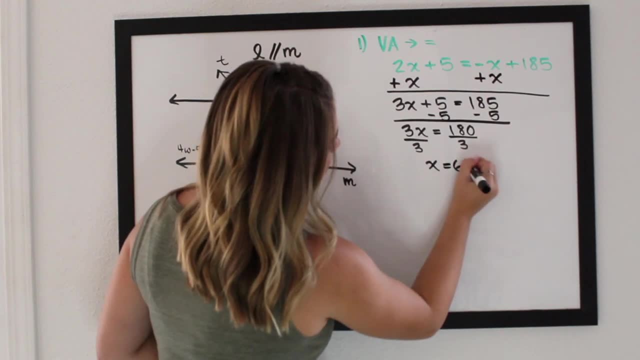 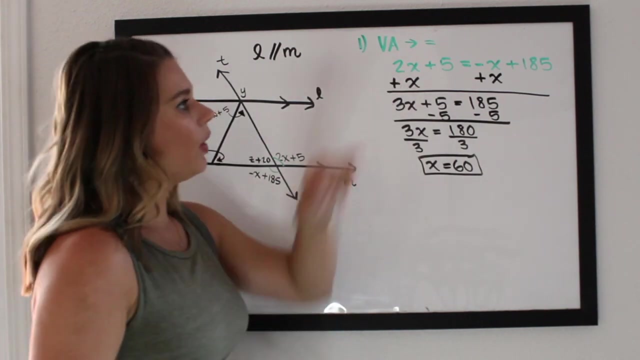 I end up with: 3X is equal to 180.. Divide both sides by 3.. X equals 60.. So step 1, identify your theorem that you're using. Step 2, set up your equation And then step 3, solve. Okay, so the 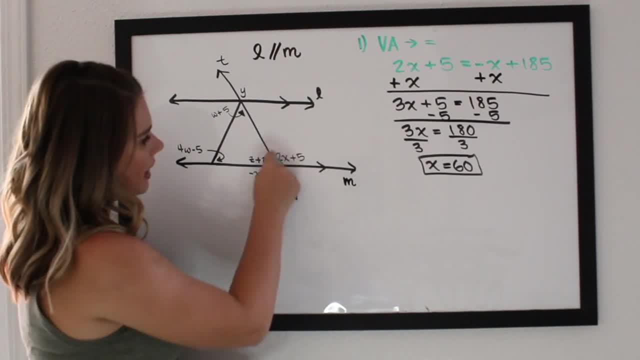 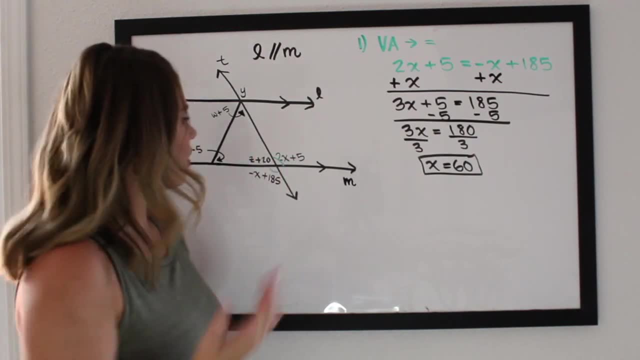 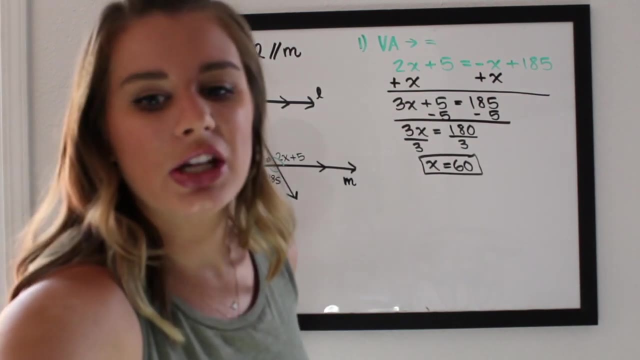 next thing that I'm looking at is: I see this 2X plus 5 and this Z plus 20, these angles right here, those angles are actually supplementary. They form a line. In other words, they're going to add up to 180 degrees. So I'm going to use that fact to set up my next equation. 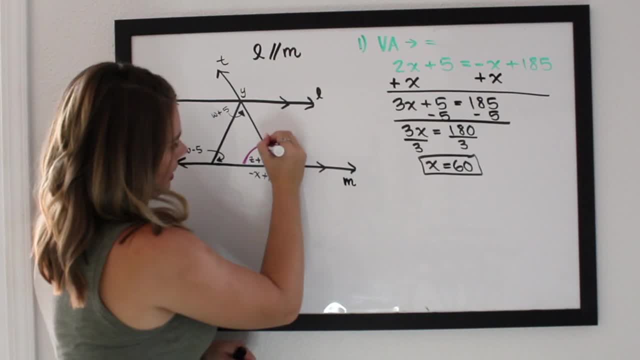 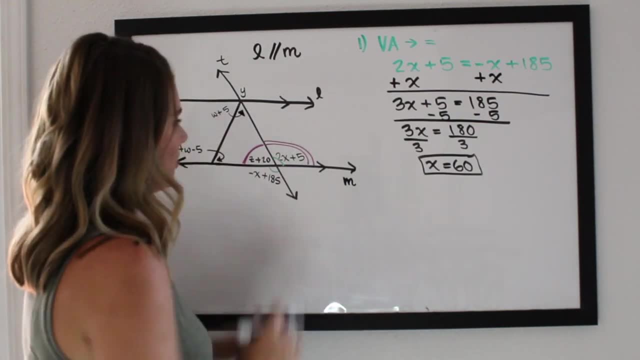 So I have this angle right here. okay, and this one right here. Sorry, I'm making it so big, I just don't want to write over the actual variables we have going on. So my second equation: we're going to use the fact that we're going to add up to 180 degrees, So I'm going to 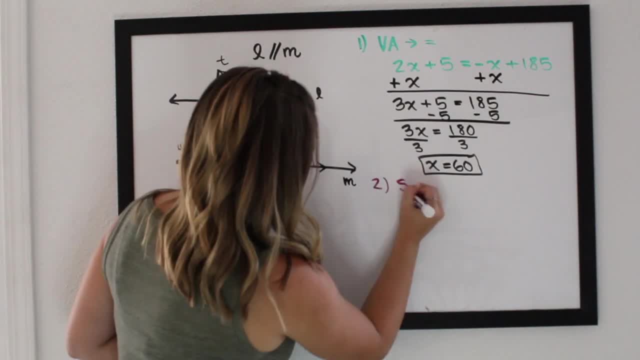 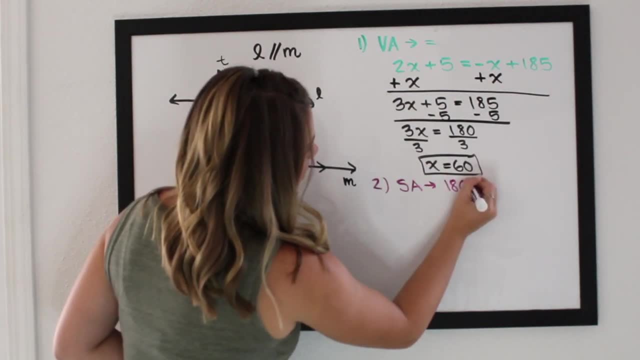 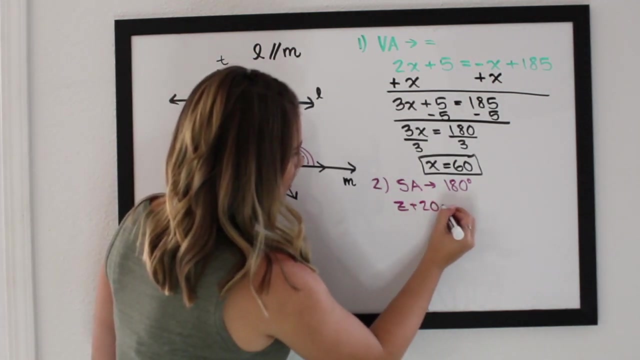 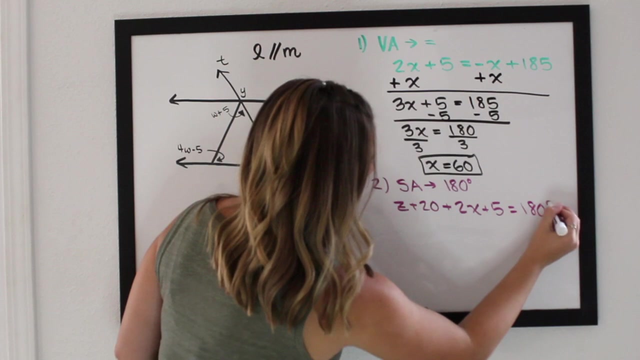 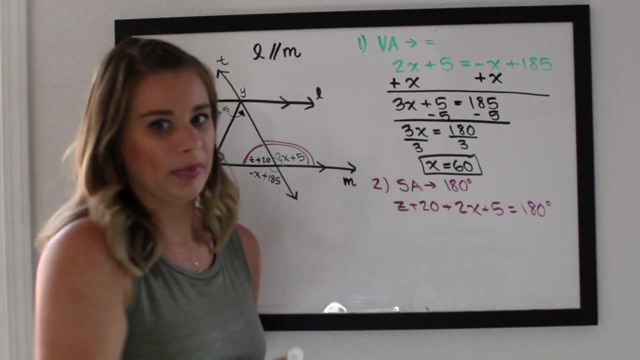 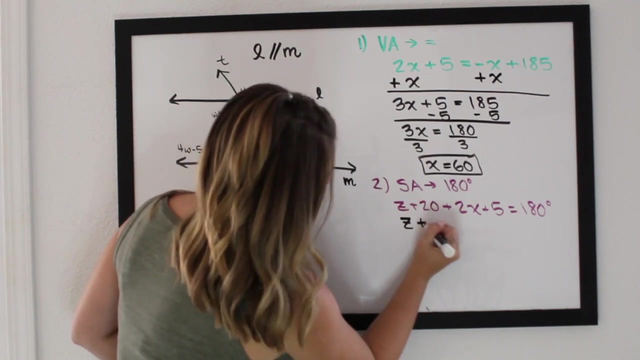 add up to 180 degrees. So that means that Z plus 20 plus 2X plus 5 equals 180 degrees. Okay, so let's clean this up. We'll combine some like terms. I have a Z- Oh, I'm going to do this in black so you can see it better. So I have Z plus 2X. I can't combine. 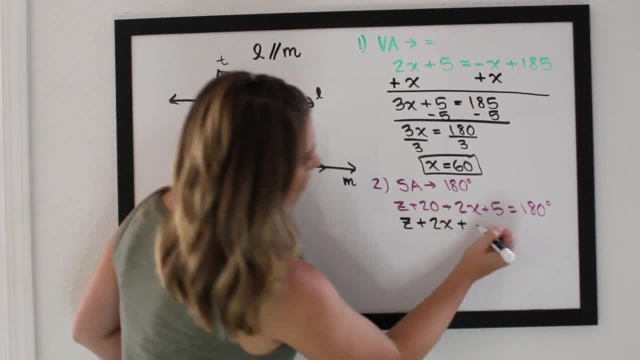 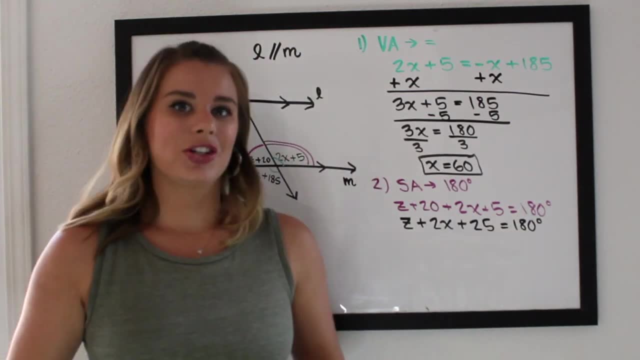 those because they're not like terms, But I can add the 20 and the 5 together. So plus 25 equals 180 degrees. Now the next thing is: I do already know what X equals. X equals 60. So I can just 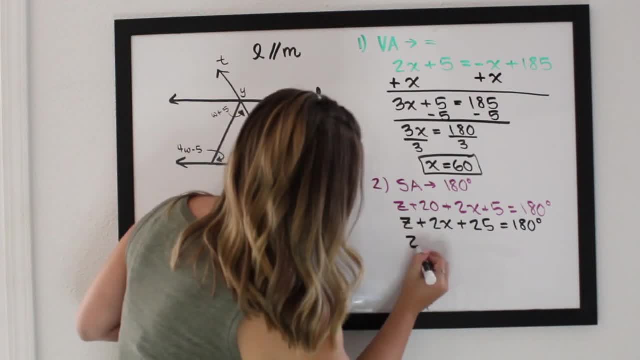 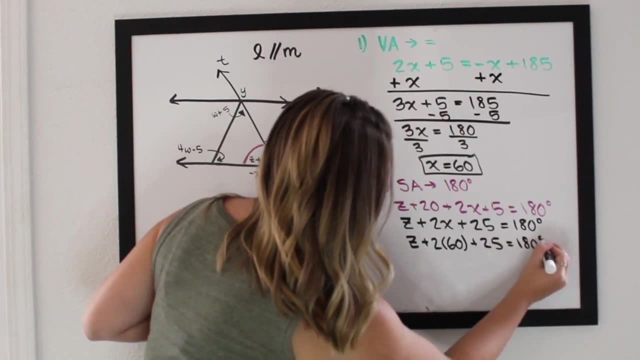 plug 60 in for X here, So then I have Z plus 2 times 60. So I can just plug 60 in for X here. So I have Z plus 2 times 60. plus 25 equals 180 degrees. 2 times 60 is 120.. So I have Z plus 120. 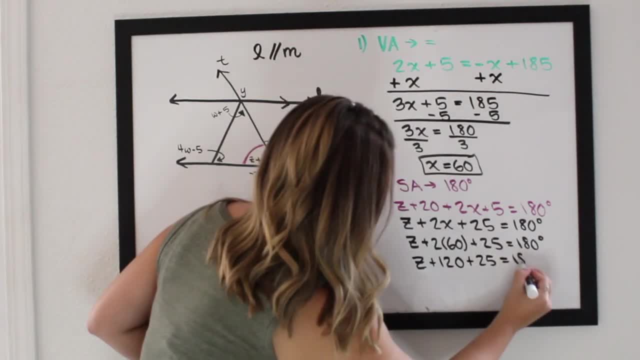 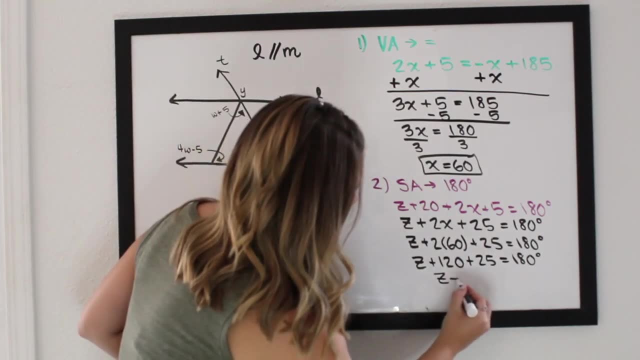 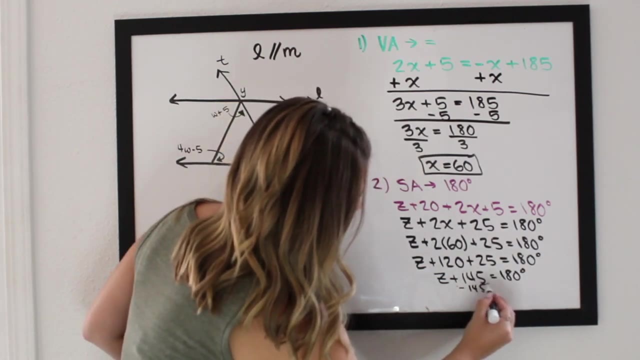 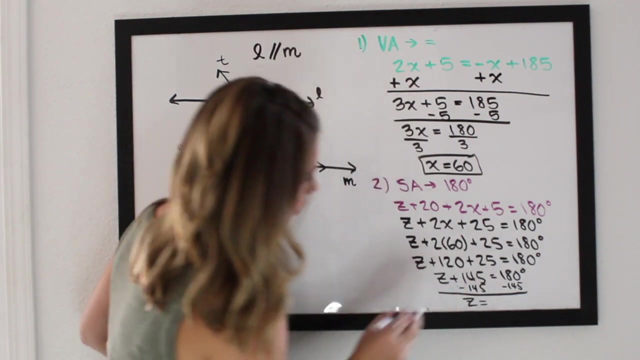 plus 25 equals 180 degrees. 120 plus 25 is 145. So I have Z plus 145 is equal to 180 degrees. I can subtract 145 from both sides, Okay. and then let's see I have Z is equal to okay. so I have 180 subtract 145. So it looks like. 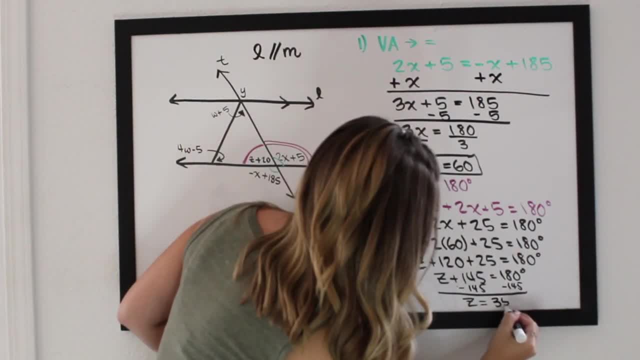 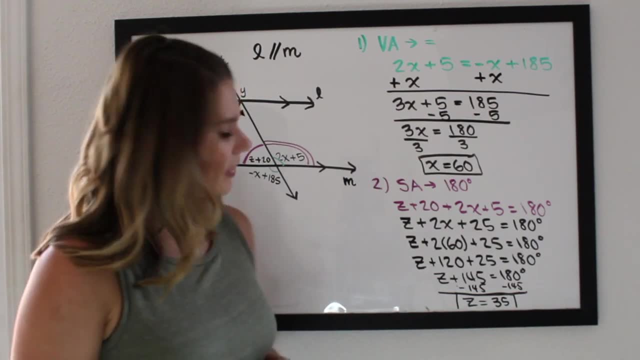 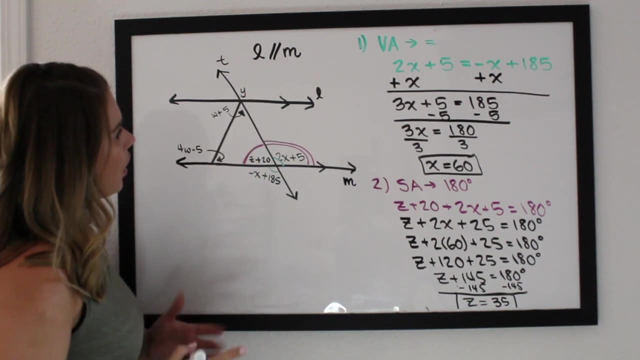 I have 35 for Z. Okay, the last variable we need to solve for just looking at our diagram here, Oh, actually we have a Y too, So let's actually do Y Next. So we need four equations. I was misspoken on that. So we need four equations because I 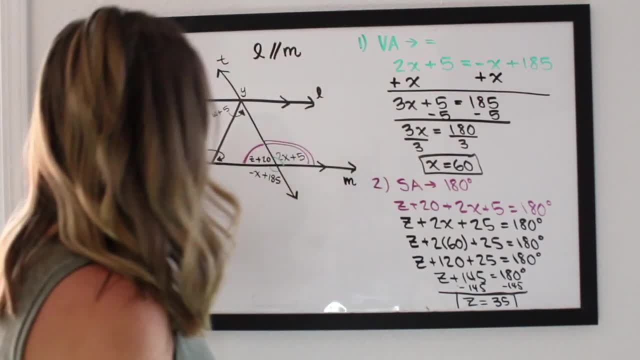 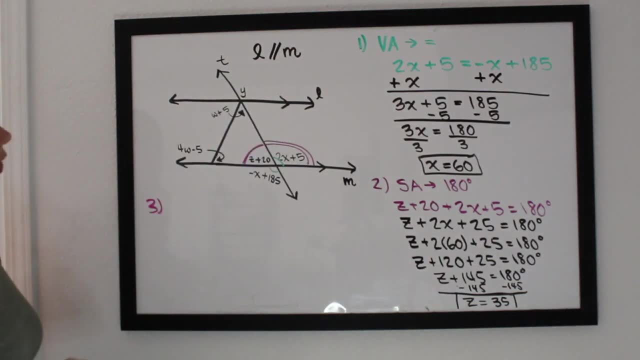 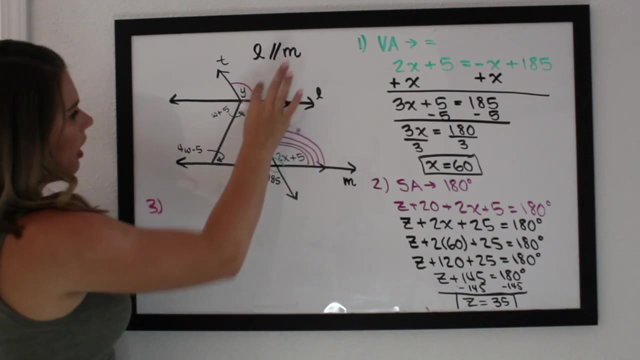 didn't see that Y up there, So I'm going to actually solve for Y now. I'm going to do this over here. So, number three: I need to solve for Y. What I have here is some corresponding angles. Okay, they're both on top of line L and N. They're on the same side of the transversal. 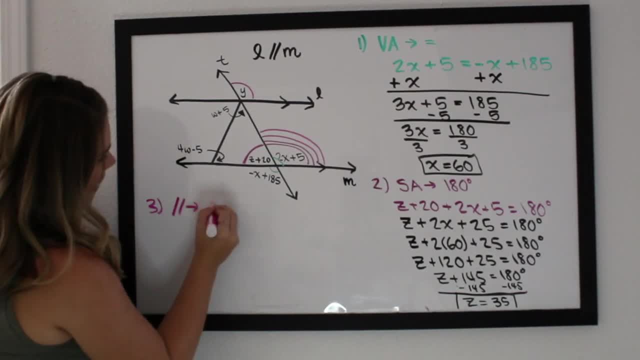 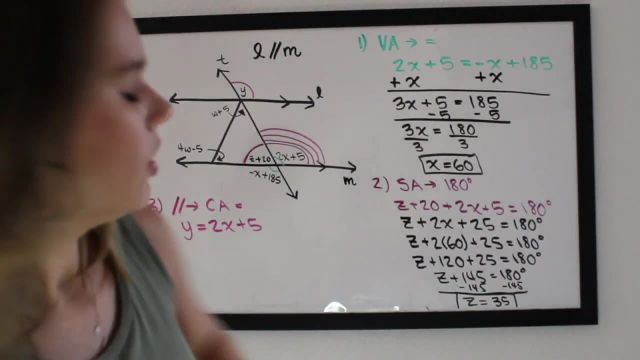 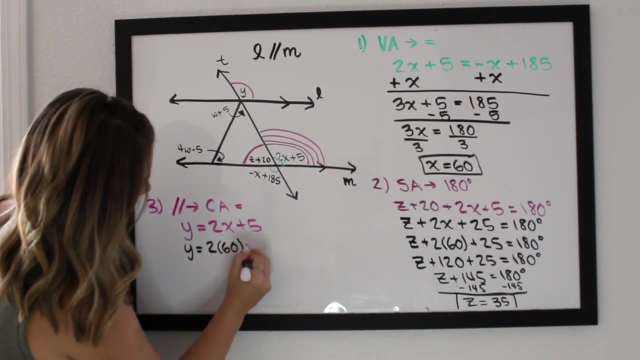 So when the lines are parallel we know that corresponding angles are equal. So for our equation, Y is going to equal 2X plus 5.. Now the nice thing is we have already solved for X, So we have: Y is equal to 2 times 60 is our X plus 5.. 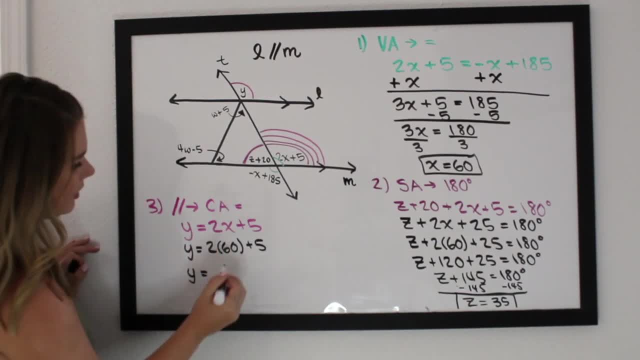 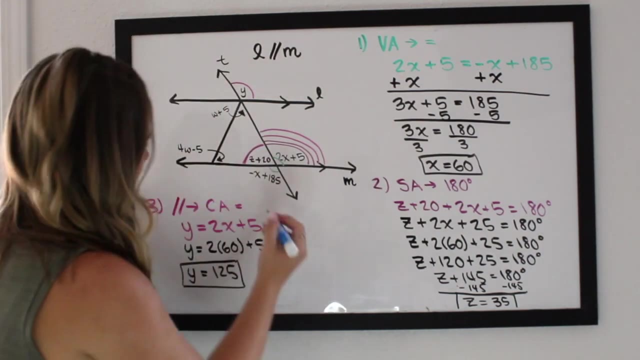 So Y equals: 2 times 60, is 120 plus 5 is 125.. All right, now we are at our last variable, which is W. So let's see. So you use what color? I might not use blue, it looks like. So number four. sorry, these are all out of order. 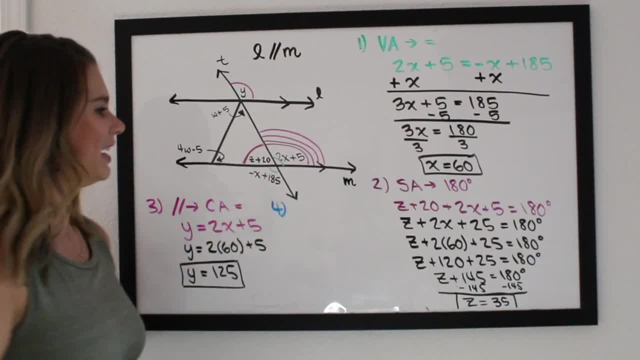 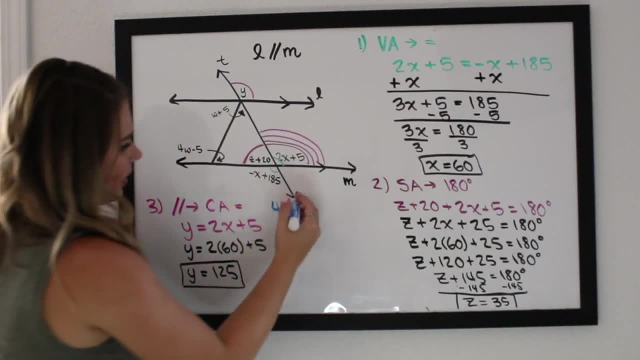 I might. I'll leave those there. I think I have enough room. Okay, so now it looks like I have a triangle here, So we can use the theorem that triangle. the sum of the angles in a triangle add up to 180.. 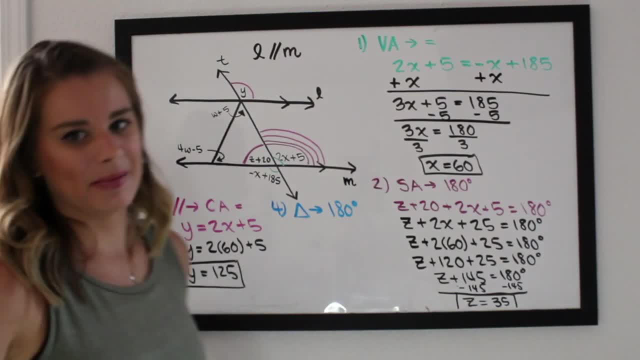 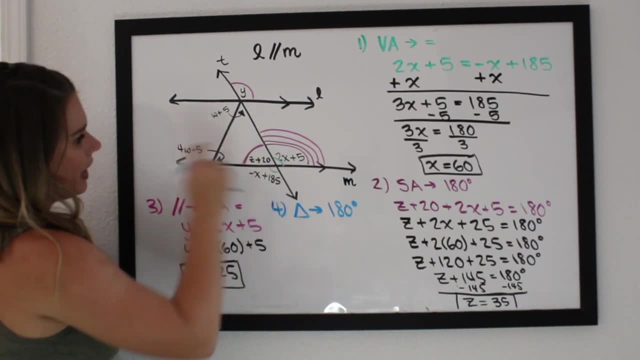 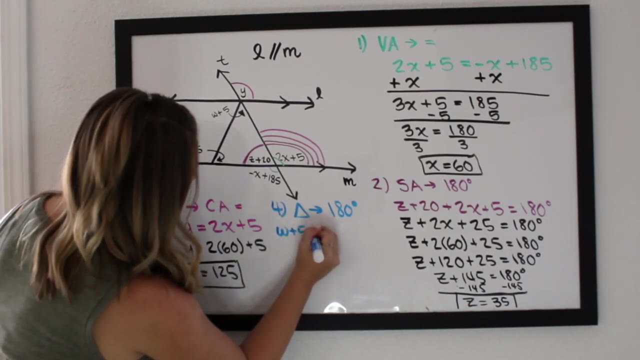 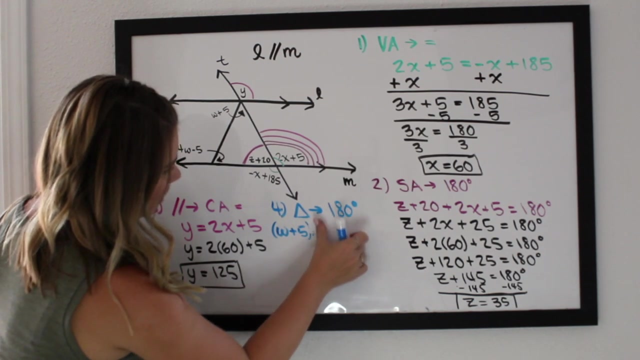 180 degrees, And I might actually run out of room here. Well, let's see. Okay, so that means this angle plus that angle plus that angle is going to equal 180 degrees. So I have w plus 5 plus 4w. Now put these in parentheses because you don't want to mix up your negatives when you're 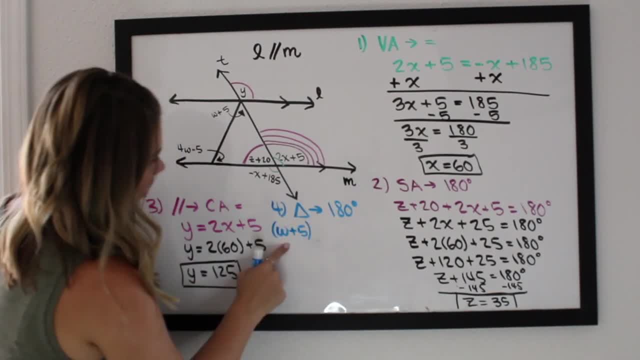 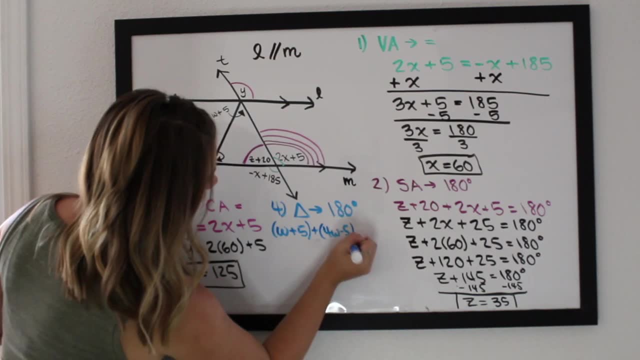 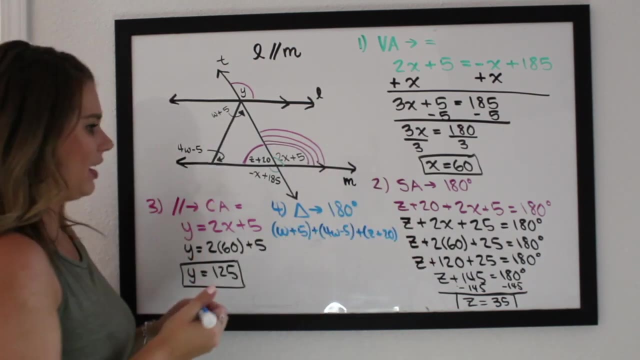 solving. Let me just rewrite that a little nicer for you: w plus 5 plus 4w minus 5 plus z plus 20 is going to equal. see, I did run out of room, So if you need those, still go ahead and rewind. 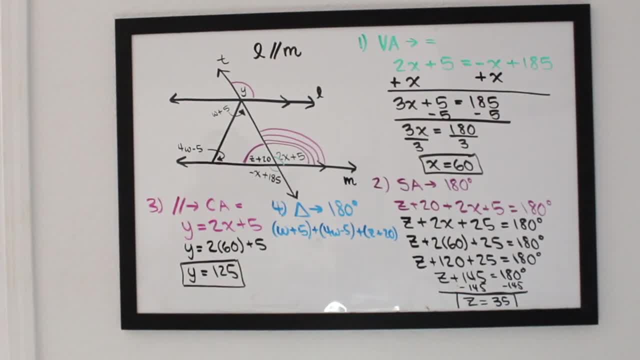 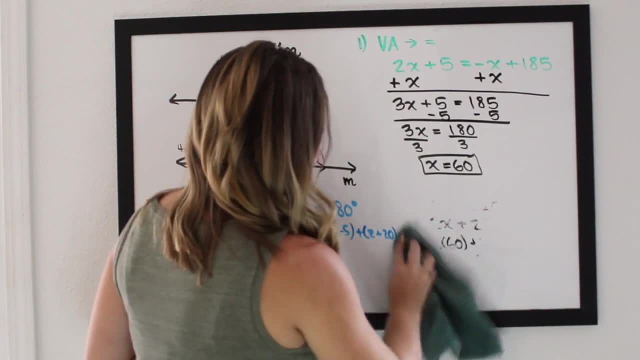 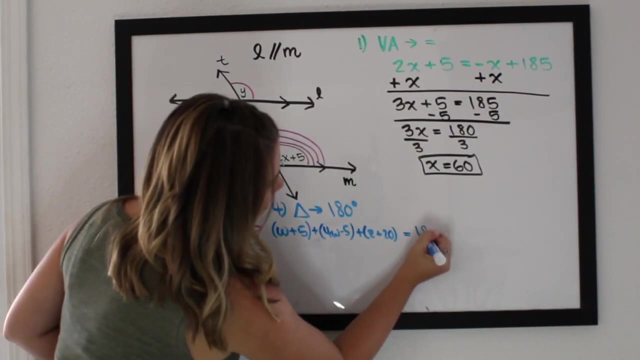 pause and you can still get those, But it looks like I do need to erase at least this one So that I have some room. Okay, sorry about that, I thought I can make it fit. So equals 180.. That's using our triangle sum theorem. Okay, so let's combine some like terms and. 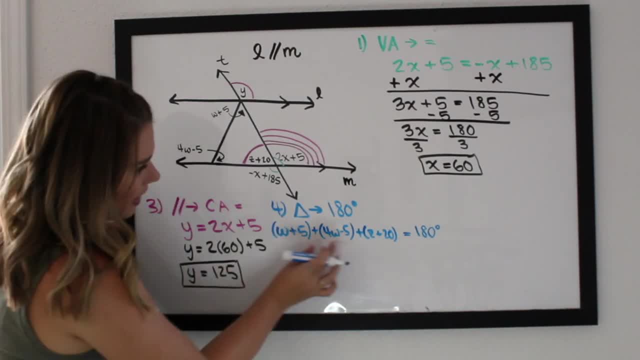 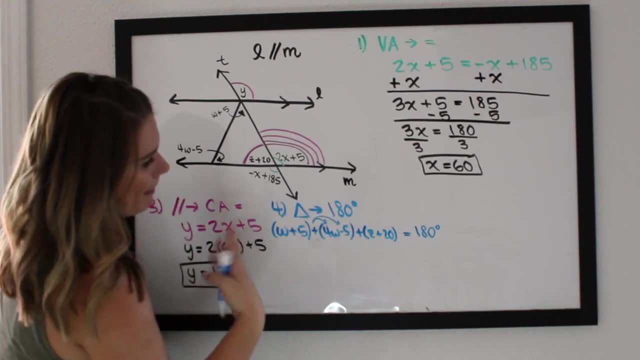 clean things up a little bit. So we have w plus 5 plus 4w minus 5.. So, remember, you kind of have to distribute this, So it's still going to be a minus 5.. Just be careful about that. So we have w plus 5 plus 4w minus 5.. So, remember, you kind of have to distribute this, So it's still going to be a minus 5.. Just be careful. 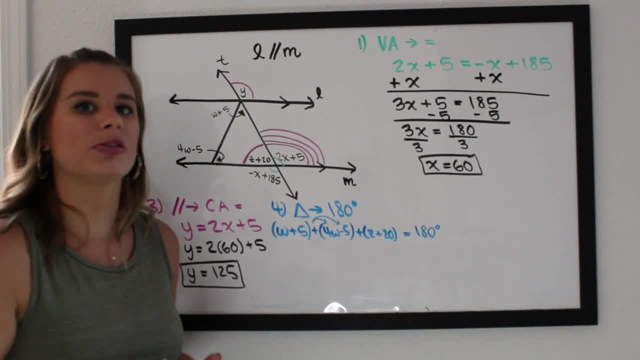 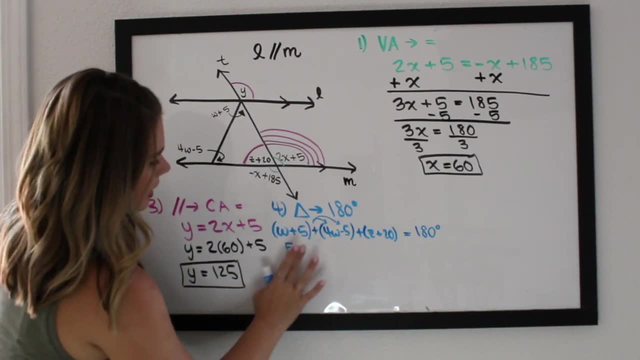 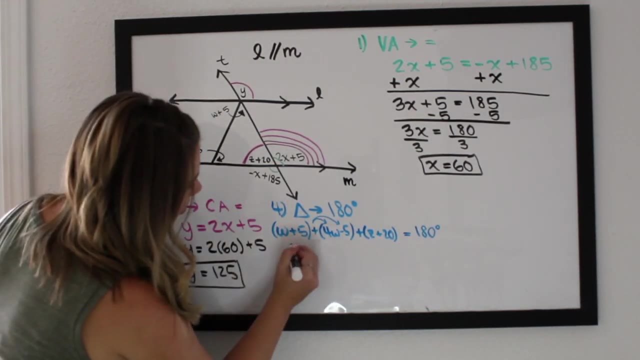 with that. Sometimes, when you're subtracting here, a lot of students forget to distribute the negative. So I have w plus 4w, So that's 5w, And let's once again, let's switch to black, just because on camera it shows up a little bit better, So you can see all my solving steps. So 5w plus. 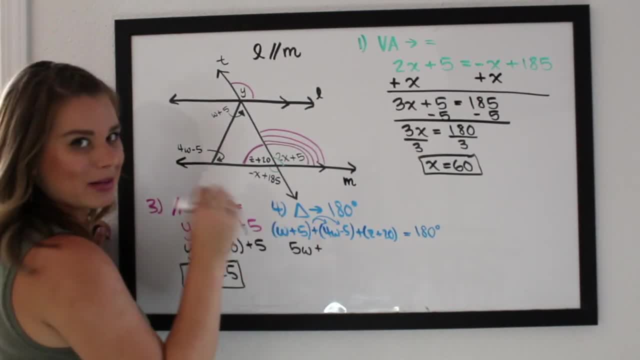 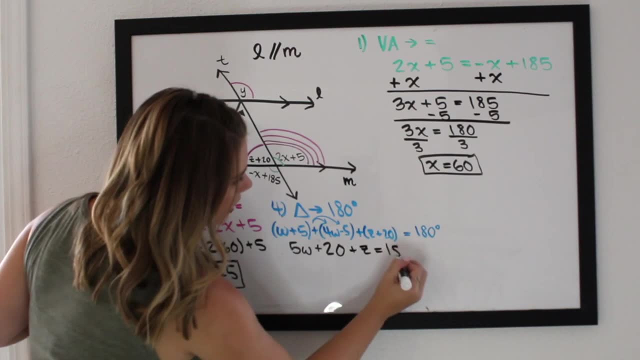 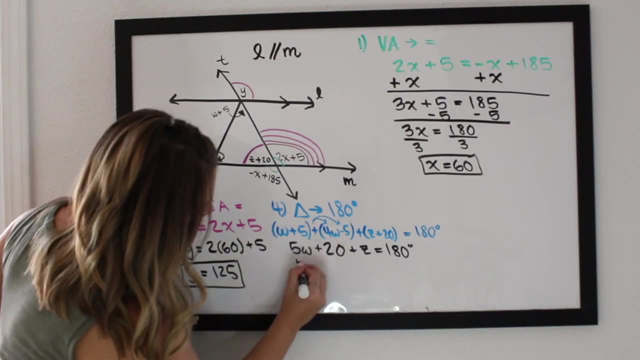 okay, so I have a plus 5 and a minus 5.. That's going to be 0, right? And then I have plus 20 plus z equals 180 degrees. Well, we also did already solve for z. I believe it's 35. So I can plug that in. So I 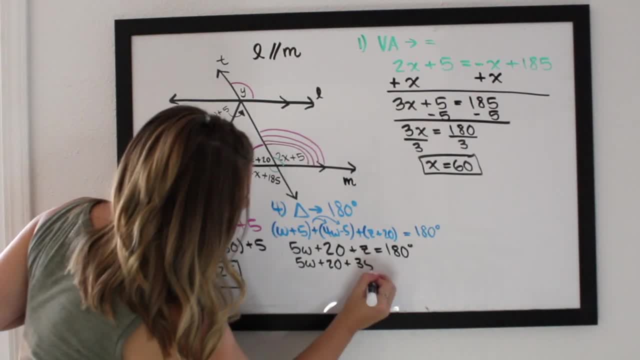 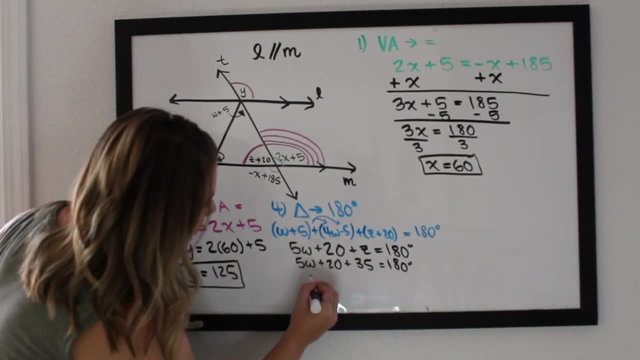 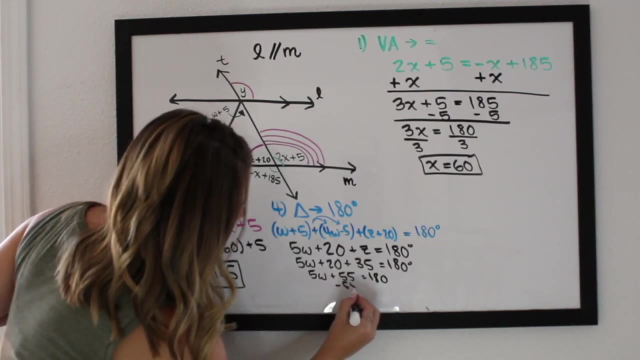 have: 5w plus 20 plus 35 is going to equal 180.. So 20 plus 35 is 55.. So I'll have: 5w plus 55 is equal to 180.. We're going to subtract 55 on both sides, Okay. 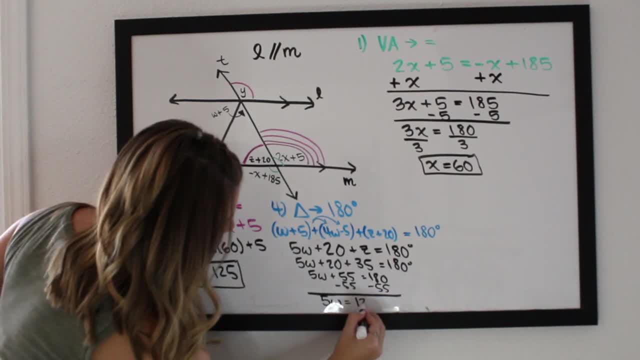 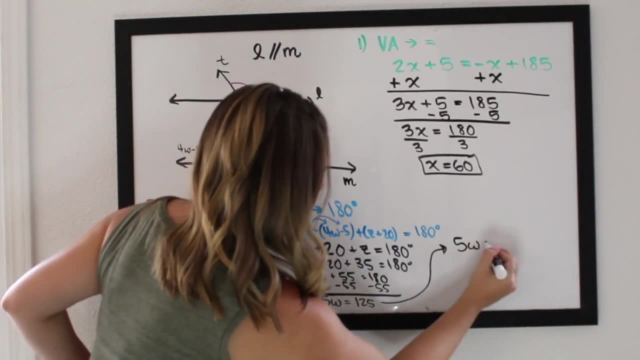 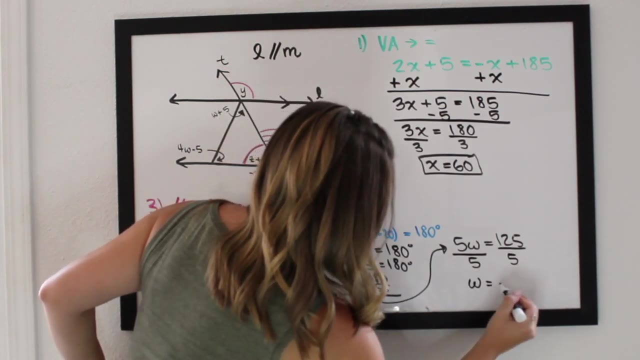 so then I have: 5w is equal to 125.. Okay, I'm going to move this up here, just so you can see that. So 5w equals 125.. Okay, divide both sides by 5.. W equals. let's see we have: 5 times 20 is 100.. 5. 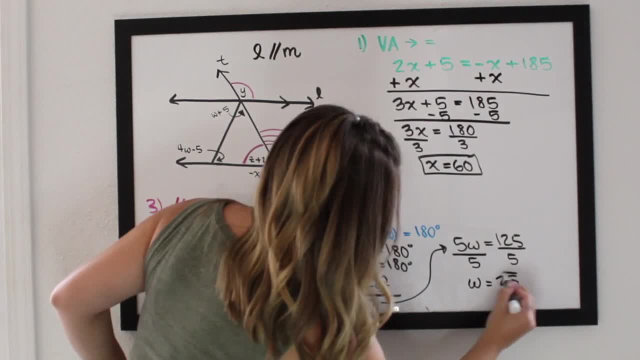 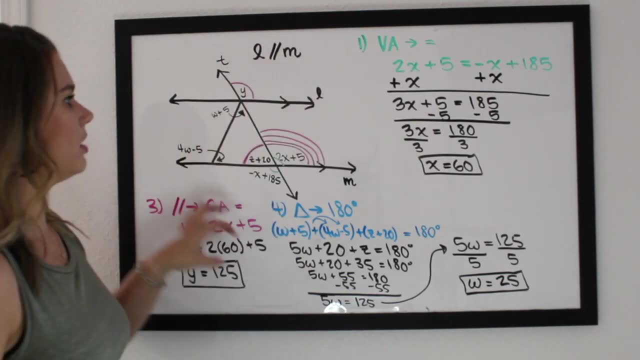 times 5 is 25.. So we have 25.. Okay, and using our angle, so we have: 25 minus 5 equals 17,. so 20 times 5 equals 50, is equals. so we have: 5 times 15 is: 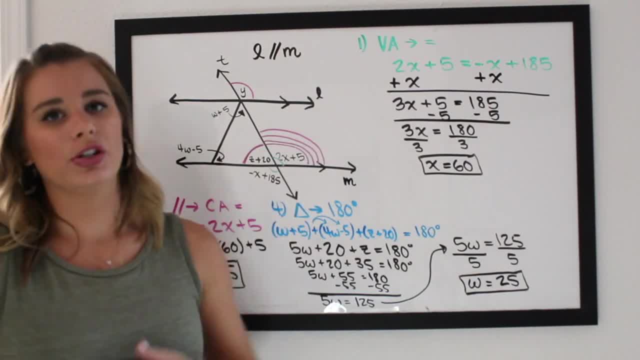 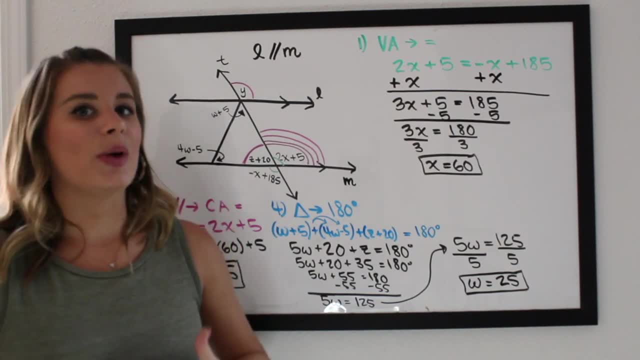 equal to 1.. Okay, so that's 325.. Okay now, in order to solve for the king of all relationships, we were able to solve for all variables in this diagram. So just remember the key points here. Step 1 is you always tell your reader what theorem you're using. Step 2 is you come up with your 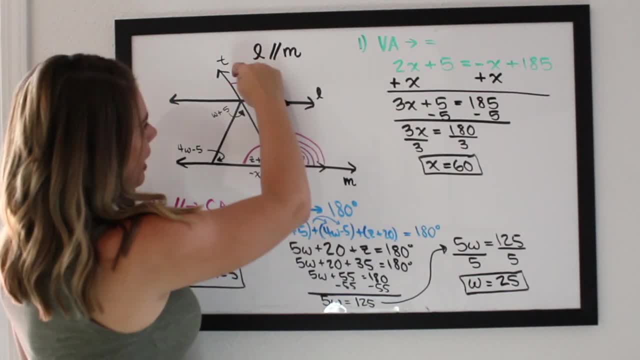 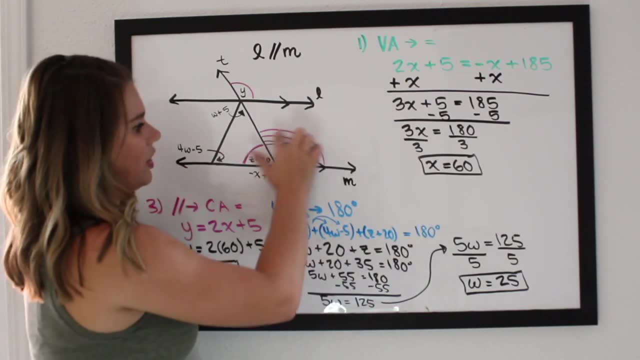 equation, And then step 3 is solve. Now you have to make sure that you answer the question that's being asked of you, whatever you got for x, for example, to find the measure of this angle. So just be careful on problems that might ask you to do that at the end. Okay, and that's all for today.